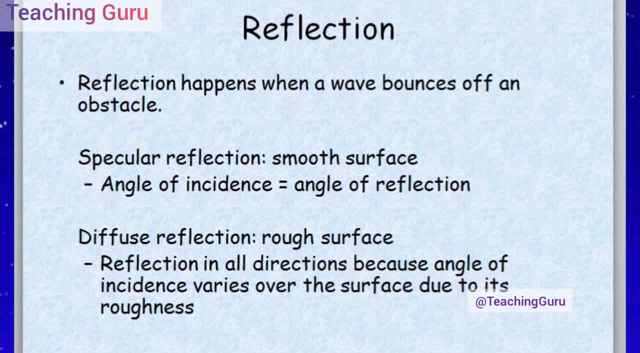 that is specular reflection and second one is diffuse reflection. First specular reflection happens on smooth surface and in this reflection angle of incidence is equal to angle of reflection. and the second one is diffuse reflection That happens on the rough surface, In this angle of incidence not equal to angle of reflection, Reflection in all direction because the angle 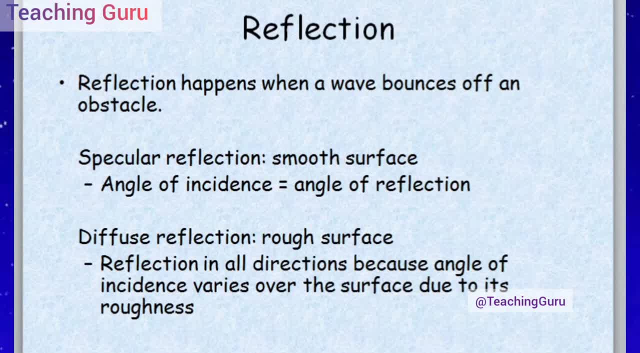 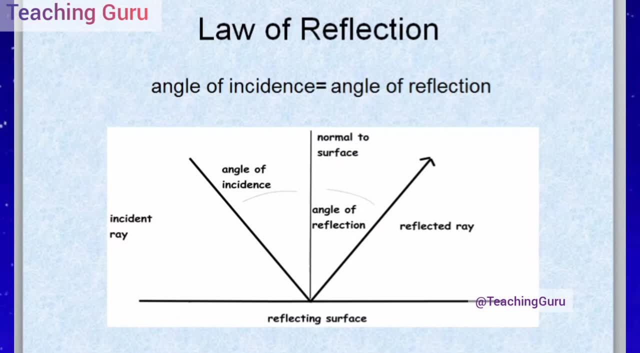 of incidence vary over the surface due to its roughness. Okay, So what is the laws of reflection? Law of reflection is the angle of incidence is equal to angle of reflection that is normal to the surface. Okay, Here, that is the incident ray and that is the refracted ray. When the 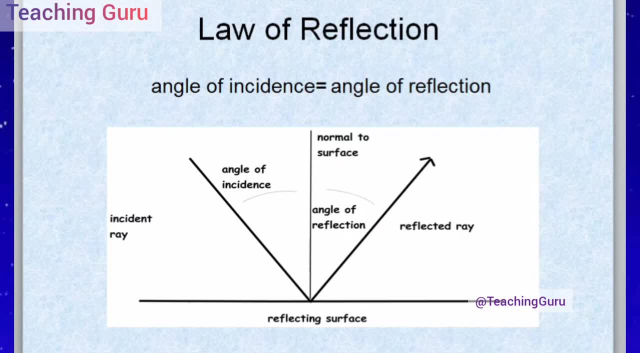 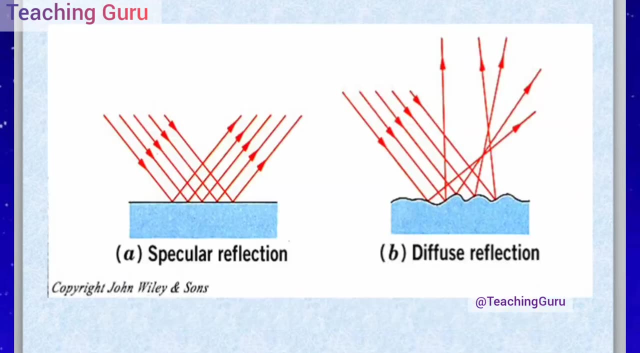 ray strike that reflecting surface and rebound back with the same angle at which the ray was incident. Okay, Here, angle of incidence is equal to angle of reflection, And this is the normal to the surface. Okay, The next one, that is, the specular and diffuse reflection. This is the example. okay, The specular reflection. and 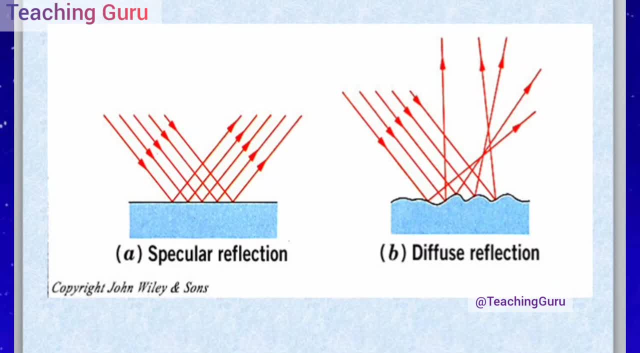 diffuser in the specular reflection. these are uniform. you can see in the diagram and in this ray. in this diagram the diffuse diffuse reflection in the diffuse reflection incident ray is uniform, But the refraction reflection reflected ray is different from the different is different and the angle between these are not equal. okay, 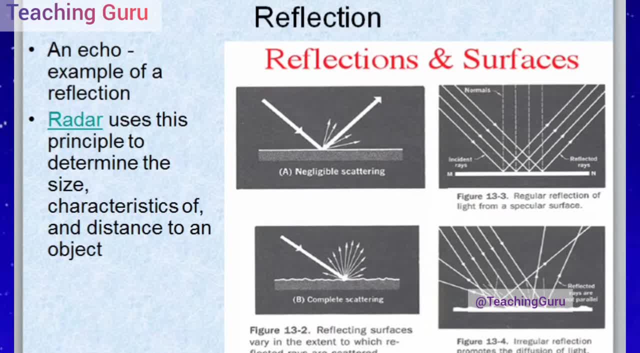 then reflection, the reflection. there are many types of reflection and many examples of reflection, like an echo. when, when you when an echo is an example of reflection, and when you speak in a- uh, blank room, in a hollow room, your sound or sound wave rebounds to the walls of the that room and 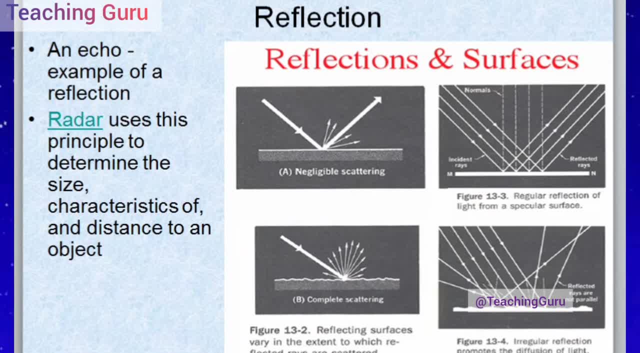 you hear the echo of your sound? okay, the echo is also example of reflection. the second one is radar radar. radar uses this principle determined to determine the size and the characteristic and distance of an object. this radar is used in many uh equipments and many defense equipments also. okay, 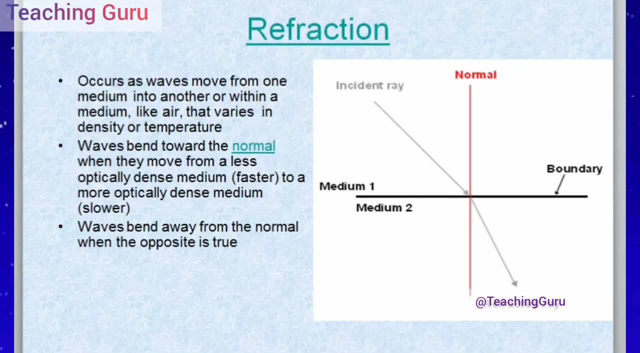 then next one is refraction. refraction occurs when waves move from one medium to another medium. the medium can be rarer or denser, both okay. so when a wave occur, when the wave move from one medium to into another or within a medium, like air, that varies in density or temperature. okay, the mother. it means that the fro there will be. 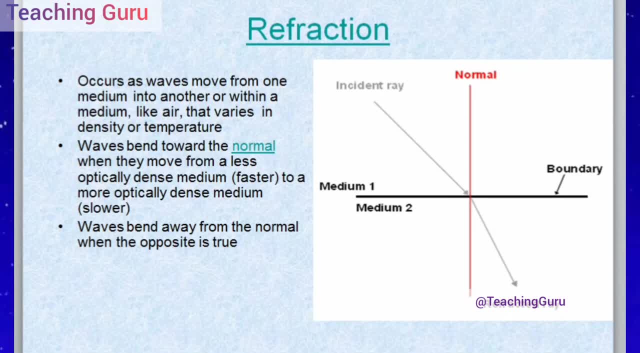 difference in density and temperature between first medium and the second medium, or incident medium or reflected medium. okay, and in this uh, in this uh process, the wave bends toward the normal when they move from denser medium to when they move from less denser medium. medium that 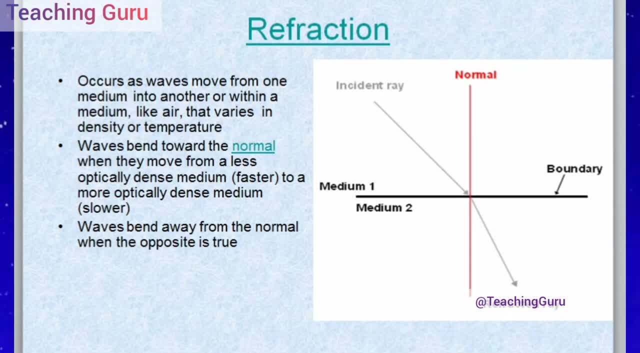 rarer medium to denser medium. this line is very important. when the ray move from rarer medium to denser medium, it it bends toward the normal. you here, you can see, and when it's a move from denser to rare, it goes away from the normal. okay, and the third point: waves went away from the normal when. 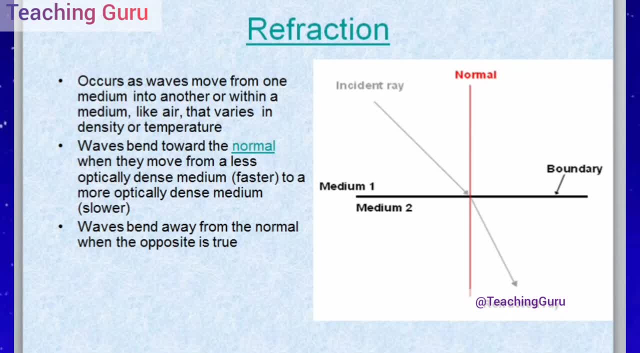 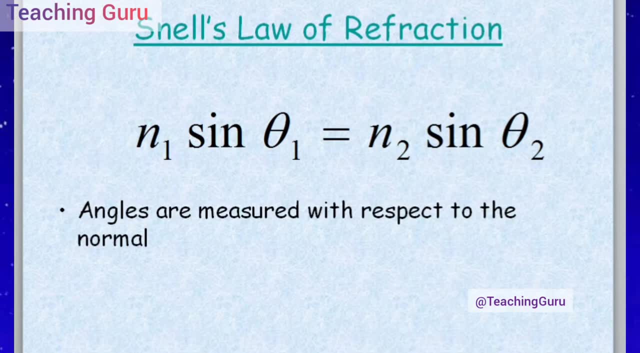 the opposite is true. okay, now let us know about the Snell's law of refraction, that is, as n 1 sine theta 1 and is equal to n 2 sine theta 2. okay, sine theta 1 is the angle, of angle, of angle between the 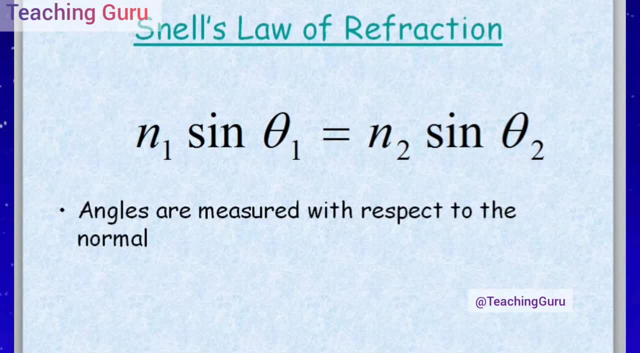 normal and the refractive incidence incident ray: okay, and one is the refractive index: okay, and one and two are the refractive index of both the medium medium 1 and medium 2: okay, and sine theta 1 and sine theta 2. that is the angle between the theta 1 is the angle between the 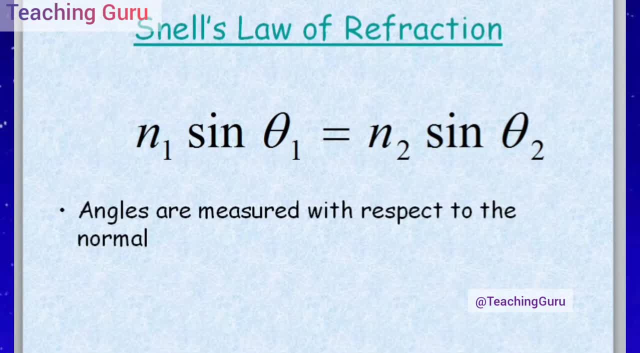 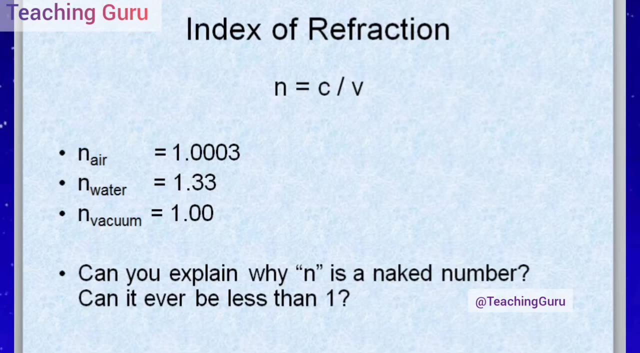 normal and the incident ray and theta. 2 is the angle between the normal and the refractory. okay, now the index of refraction, that is n, is equal to C bar V. okay, where and if, in general purpose, the refractive index of air is taken to be 1? but 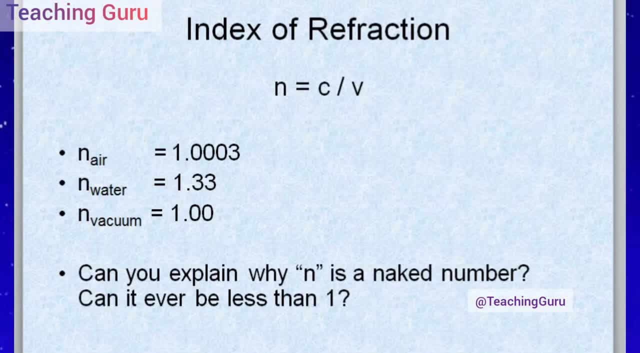 here is 1 point 0, 0, 3, and the water is 1 point 3, 3 and of vacuum is pure 1. okay, and is equal to C by V, see the speed of light, and V is the velocity of that ray. okay, 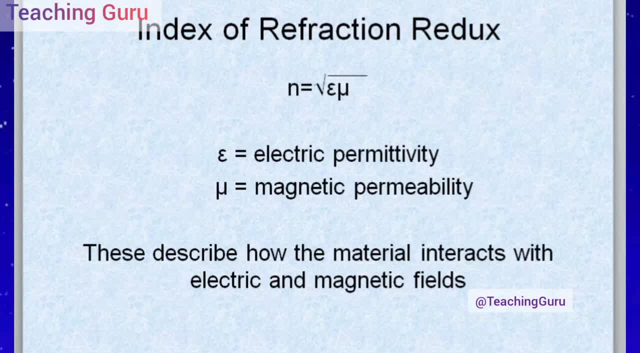 now second and second. we will go to the next slide, that is index of refraction redux. okay, n is equal to psi, u, mu, psi is equal to electrical permittivity and mu is equal to magnetic permanent. if you have learnt about electrical and magnetic field, you will you. 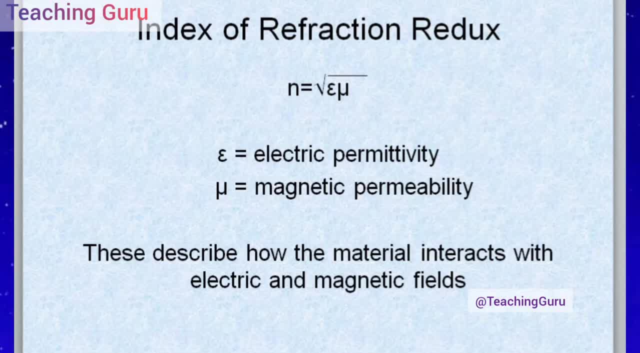 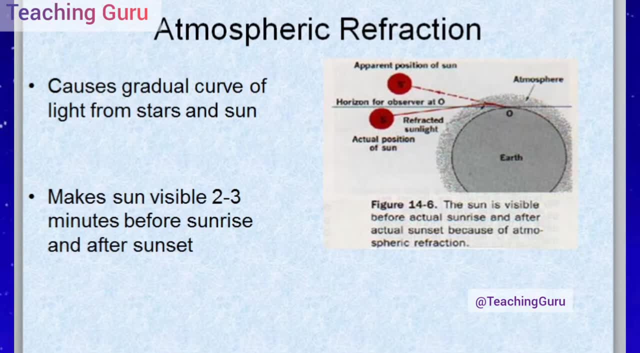 will able to understand this. okay, what is atmospheric refraction? atmospheric refraction is a gradual curve of light from stars and Sun- okay- to the earth- okay. when any the rays from the Sun in a enters our Earth's atmosphere, it bends and that is called atmospheric refraction. 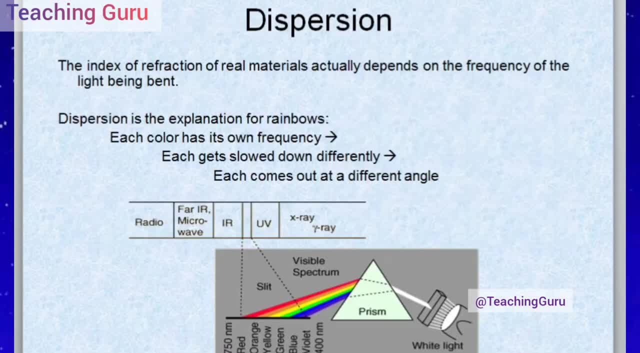 okay, and then next topic is dispersion. dispersion, the index of refraction of real materials, actually depends on the frequency of light being bent. okay, the dispersion is the example for rainbows. each color has its own frequency, each gets slowed down differently and each comes at different angle. it's the perfect example of whenever, when a white 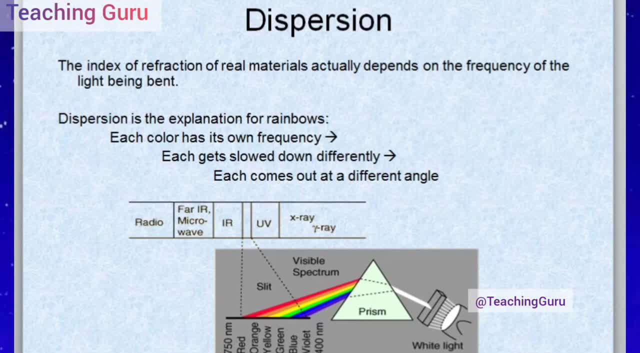 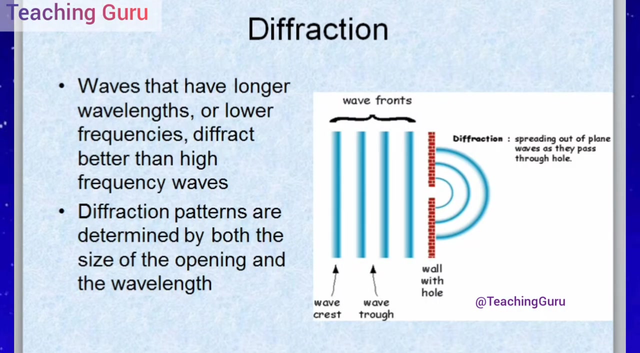 light strikes on the prison, it it splits into the bird colors with girl promise, rainbow colors. okay, this, this question can be asked. the splitting of white light in the through the prism is called what? and this is called a dispersant, okay, and the next one is diffraction, infraction, diffraction waves. 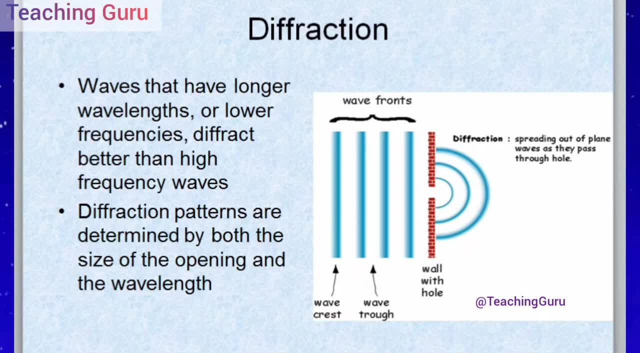 that have longer wavelengths or lower frequency diffract better than higher frequency wave. that is the rule of diffraction and the second one is diffraction patterns 나 are determined by both the size of the opening and the wavelength. okay, we are. we are supposing that you will and you are understanding this. we are only. 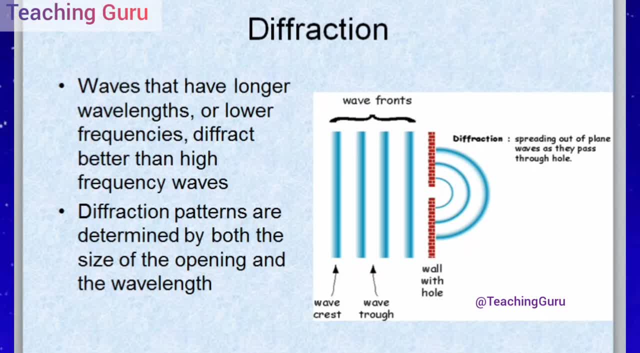 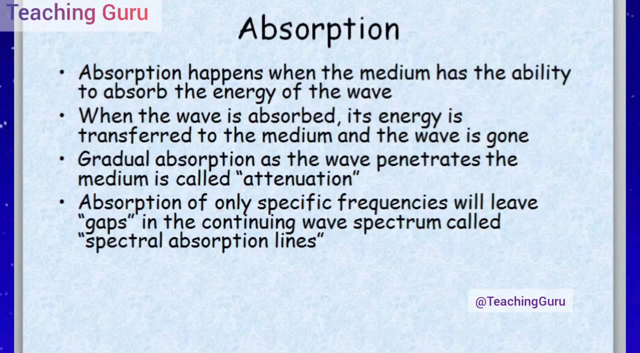 taking the quick view of this topic, so I am NOT explaining you in you this in detail. if you want to study about this in detail, there are further more videos on this channel. you can watch it, okay. and the next topic is absorption- absorption- absorption happens when the medium has the ability to absorb the 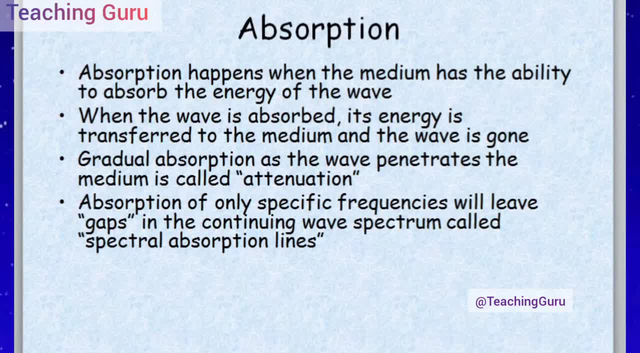 energy of the wave. when the wave is absorbed, its energy is transferred to the medium and the wave is gone. and the gradual absorption as the wave penetrates medium is called attenuation. attenuation is also called a repetition. okay, repetition of wave and the last one is absorption of only specific frequencies will leave gaps in the 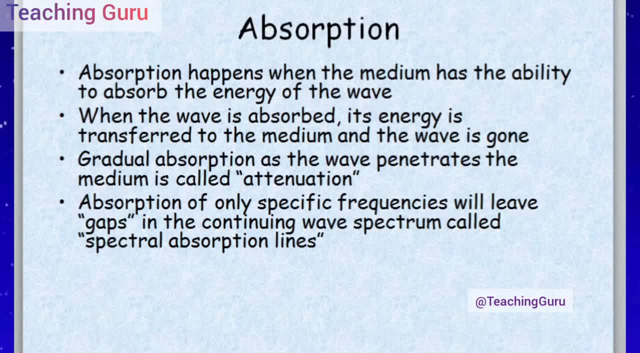 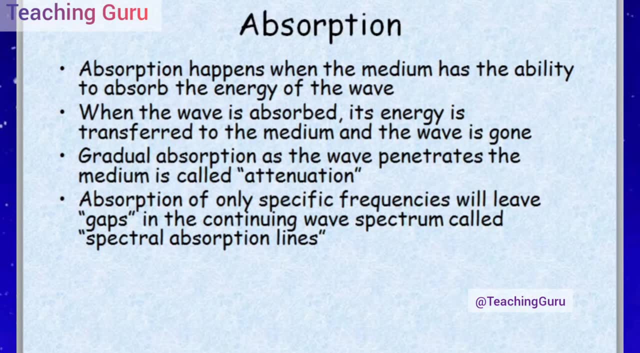 continuing wave spectrum, called spectral absorption line. okay, this line is very important for competitive exam. that is what is spectral absorption line? okay, spectral absorption line: I, as I have told you earlier that this line, this topic is very important absorption line for competitive examination, like J memes and J advance absorption line. they can ask you to the frequency of 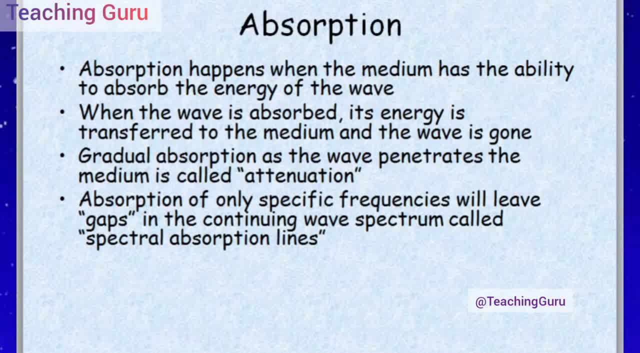 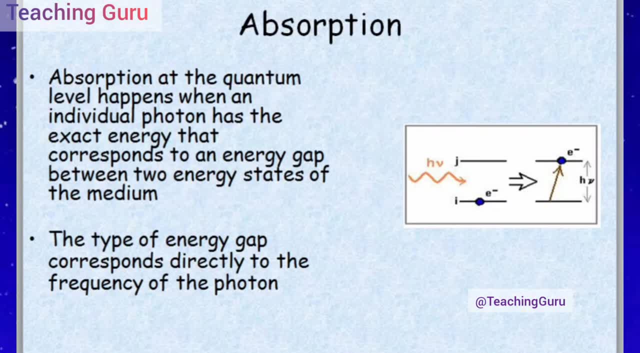 these spectral lines, okay, okay, then we will go to the next slide, that is absorption. absorption at the quantum level happens when individual photon has the exact energy that correspond to the two energy gap between two energy states of the medium, and the type of energy gap correspond directly to the frequency of photon. okay, now we'll learn about scattering. 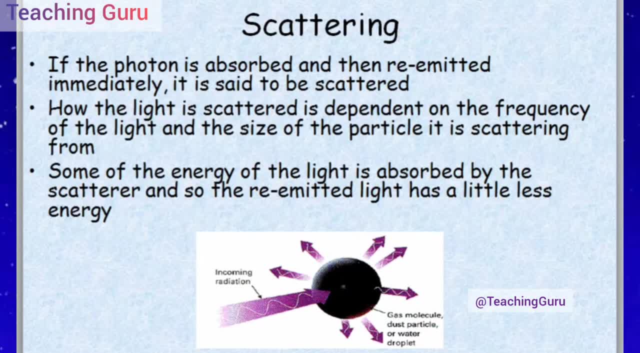 scatter. if the photon is absorbed and then re emitted immediately, it is called to be scattered or it is said to be scattered. when the light is scattered is dependent on the frequency of light and the size of particle it is scattering from. some of the energy of light is absorbed by the scatterer and the show. 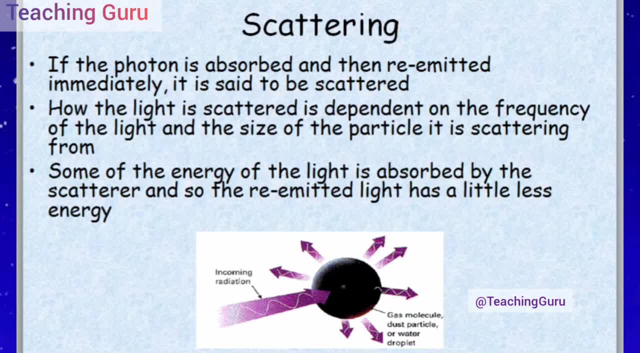 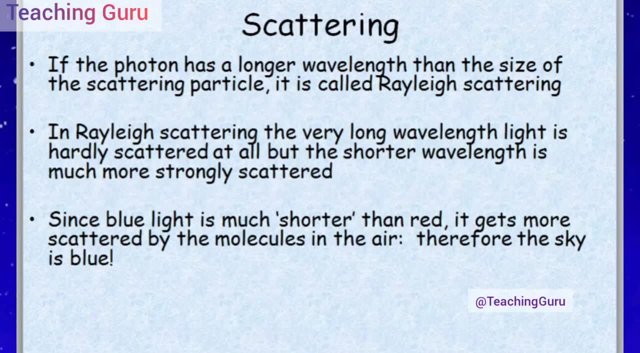 the re emitted light has a little less energy. let's know more about scattering. that is, if the photon has a larger wavelength than the size of scattering particles. this is called relic scattering, relic scattering. this point is also important, that is, please underline in your notebook, if you are. 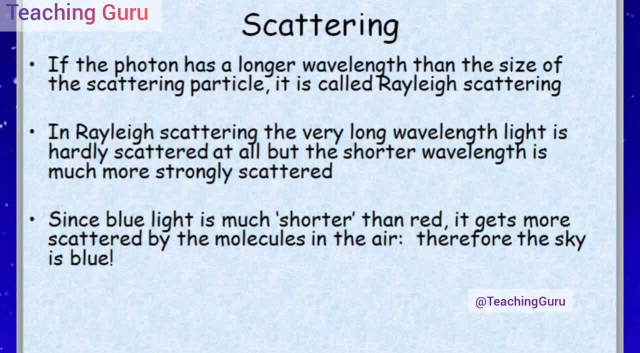 writing that relic scattering. if the photon has a larger, longer wavelength than the size of the scattering particle, then it is called relic scattering particle. it is called relic scattering. in relic scattering the very long wavelength light is hardly scattered at all, but the shorter wavelength is much more strongly scattered. since blue light is much shorter than red, it gets more. 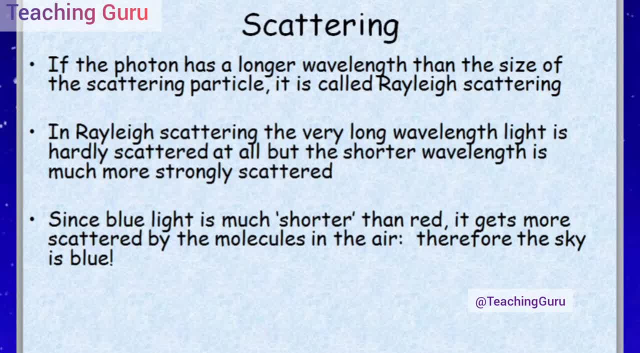 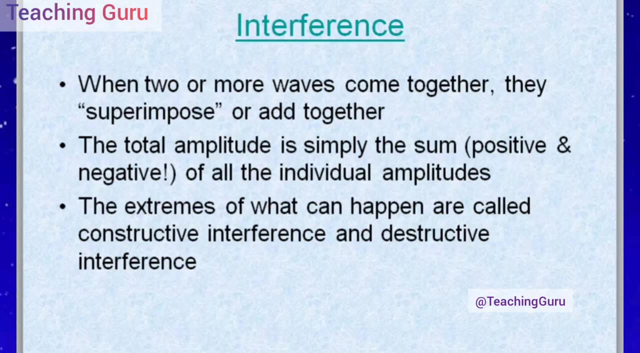 scattered by the molecules of in the air and therefore the sky is blue. and, if you know, in many traffic signal they read red, because red light very scatters, very less than the size of the scattering particles. that is why it is called relic scattering. now next topic: interference. interference when two or more waves come together. they 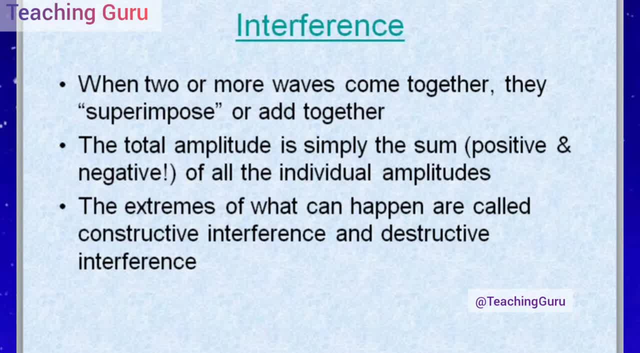 superimpose or add together. the total amplitude is simply the sum, or positive or negative, of all the individual amplitude. the extreme of what can happen are called constructive interference and destructive interference, which are very important: the constructive interference and destructive interference, and this is the example of constructive and destructive interference. 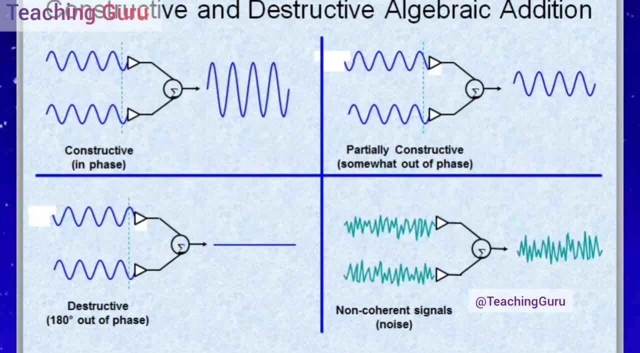 destructive algebraic addition. when two constructive waves come together in same phase, they, they form this type of wave. when two destructive wave comes in this and they, when they are in summation, this is this type of wave is formed. that is straight line. and when partially constructive and non coherent signal. 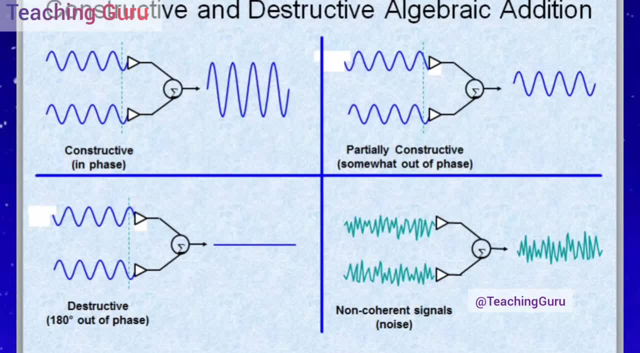 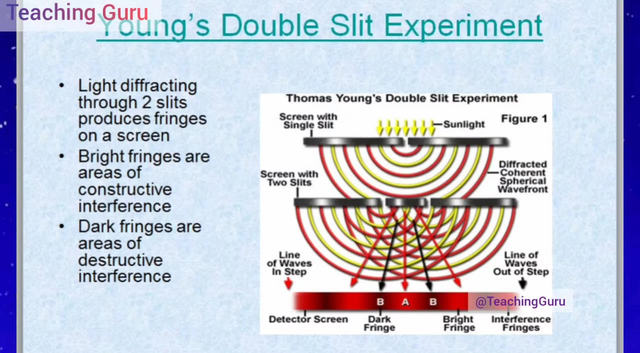 that is called noise. okay, this, this diagram, is very important for examinations point of view. now we learn about young double slit experiment. young double slit experiment is that the light diffracting through two slits produce fringes on a screen. bright fringes are the area of.